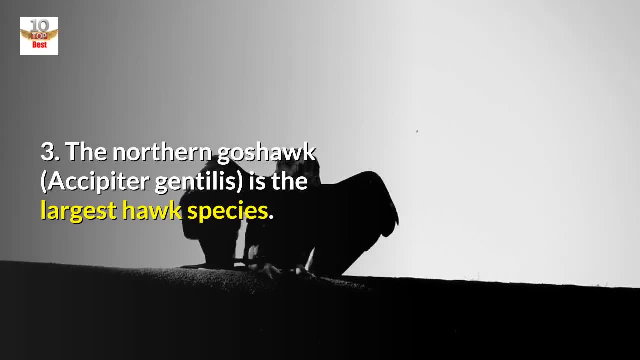 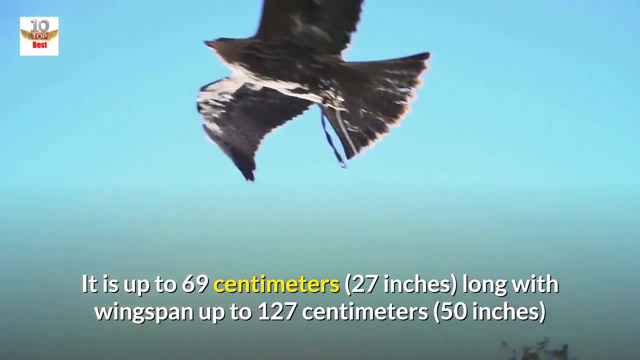 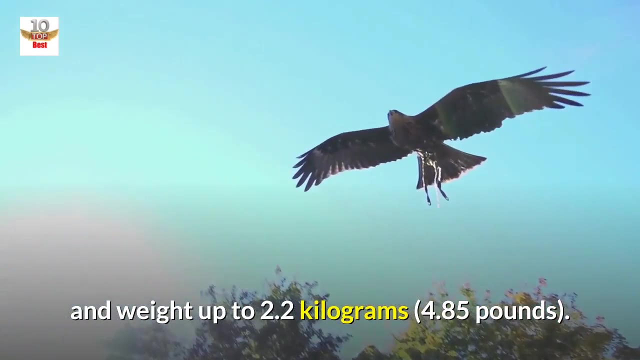 3. The northern goshawk is the largest hawk species. It is up to 69 cm- 20 cm inches long, with wingspan up to 127 cm and weight up to 2.2 kg. 4. The little sparrowhawk is the smallest hawk species. 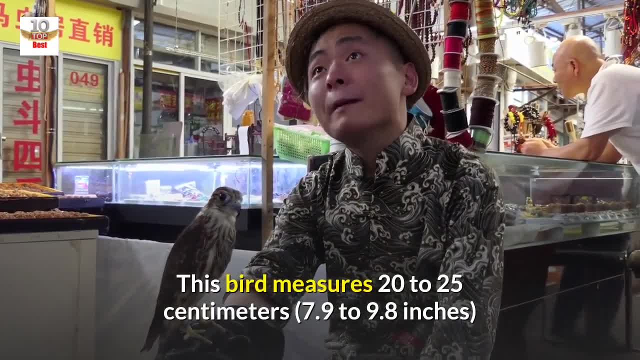 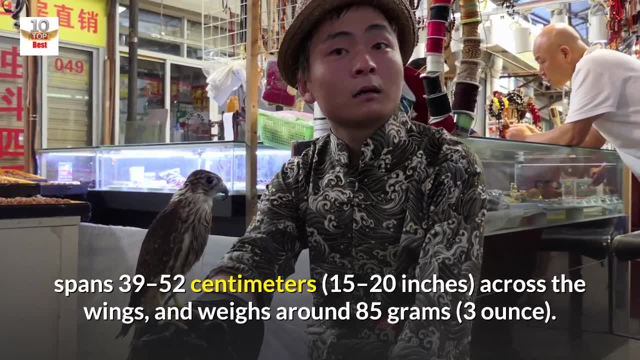 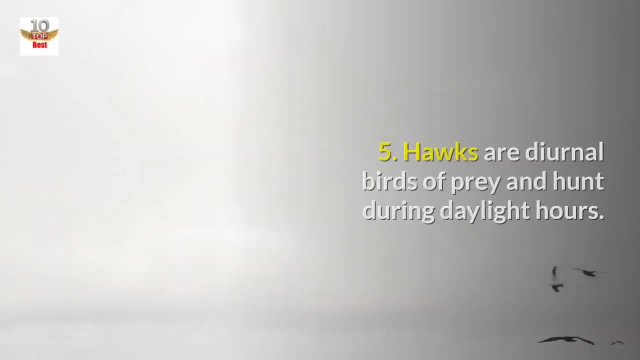 This bird measures 20 to 25 cm in length. the tail makes up about half of its length, spans 39 to 52 cm across the wings and weighs around 85 grams. 5. Hawks are diurnal birds of prey and hunt during daylight hours. 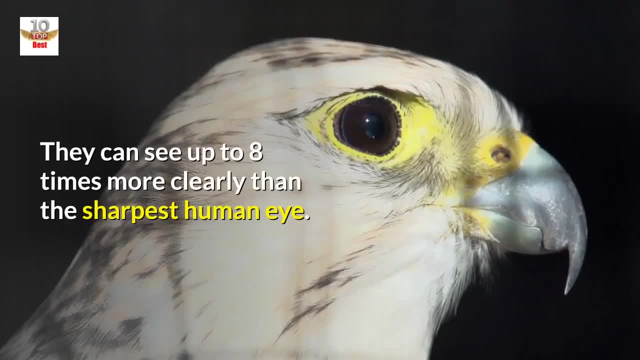 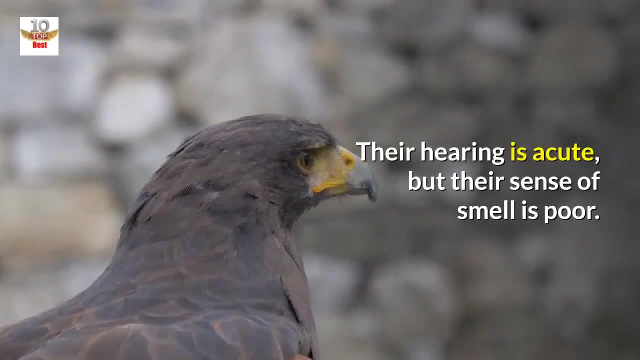 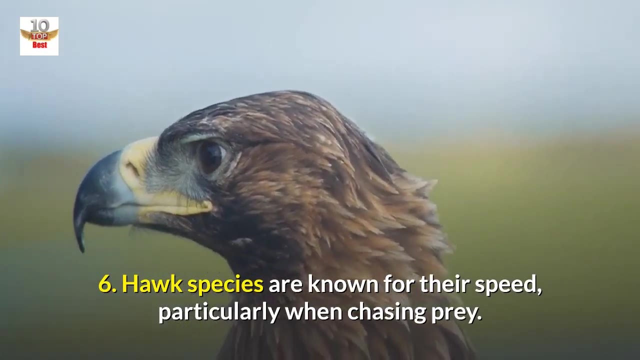 Hawks have excellent eyesight. They can see up to eight times more clearly than the sharpest human eye. Eyesight is primarily used for hunting. Their hearing is acute, but their sense of smell is poor. 6. Hawk species are known for their speed, particularly when chasing prey. 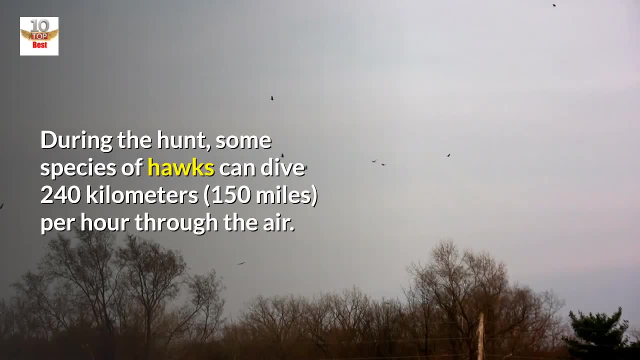 During the hunt. some species of hawks can dive 200 km per hour. Some species of hawks can dive 200 km per hour. However, the hawks' size may vary depending on their Hunger index or皮 lemps, which may differ between 60 to 90 kg. 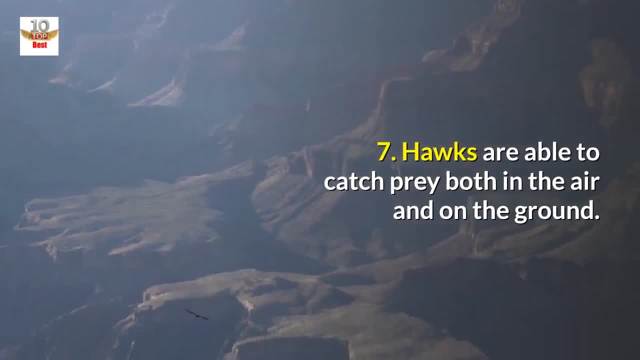 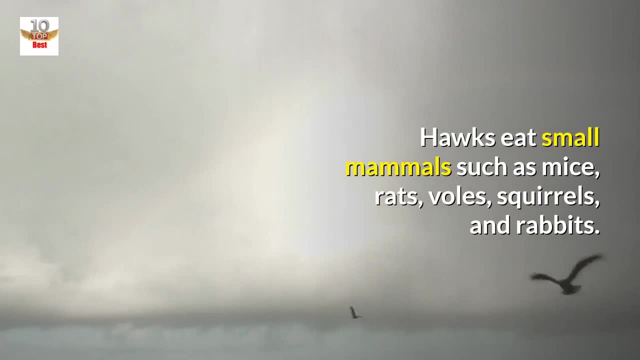 More rehearsal is required. These species sometimes rattle 7.. Hawks are able to catch prey both in the air and on the ground. They use their sharp talons to both catches and kill their prey. Hawks eat small mammals such as mice, rats, voles, squirrels and rabbits. 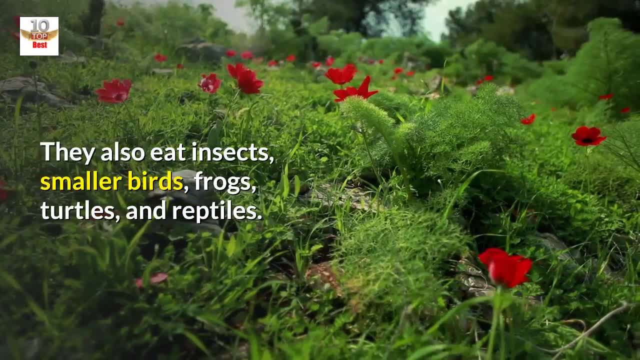 They also eat insects, smaller birds, frogs, turtles and reptiles. Some hawks will even eat snakes and crustaceans. 8. Some individuals have never eaten. in fact, Being able to grab their coffee, they will usually eat cables. 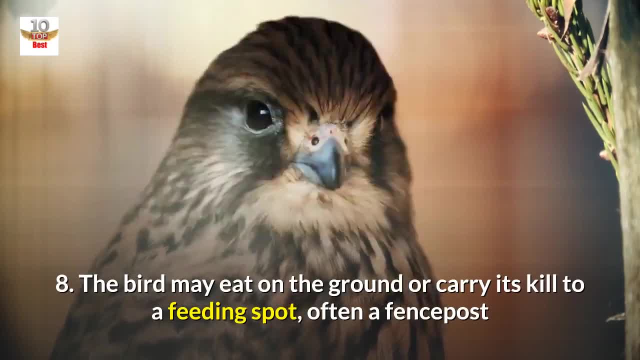 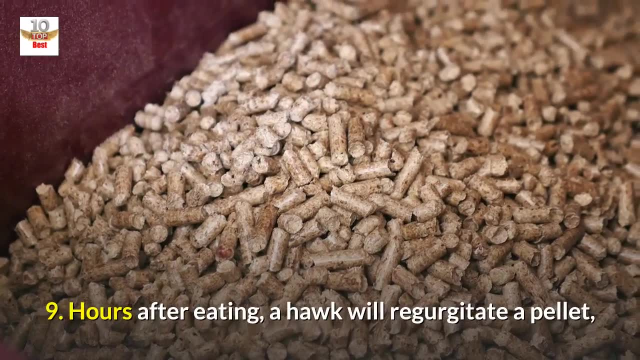 ог. It may eat on the ground or carry its kill to a feeding spot, often a fence post or tree limb, where it plucks its prey and tears the meat apart with its beak. 9. Hours after eating, a hawk will regurgitate a pellet containing any feathers, fur or 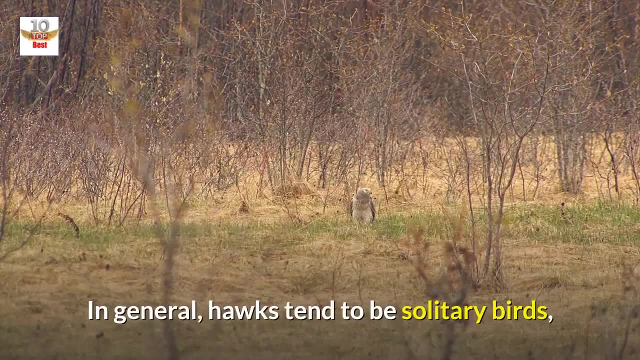 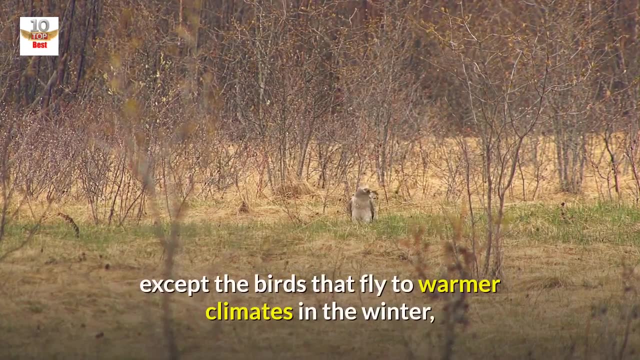 small bones swallowed accidentally. In general, hawks tend to be solitary birds, living with a mate during the spring but otherwise surviving alone, except the birds that fly to warmer climates in the winter when they create large flocks during the migration 10.. 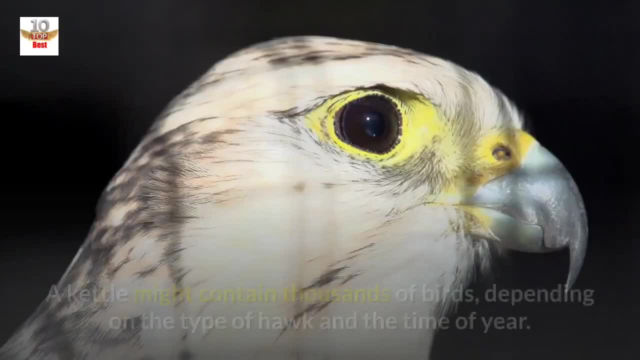 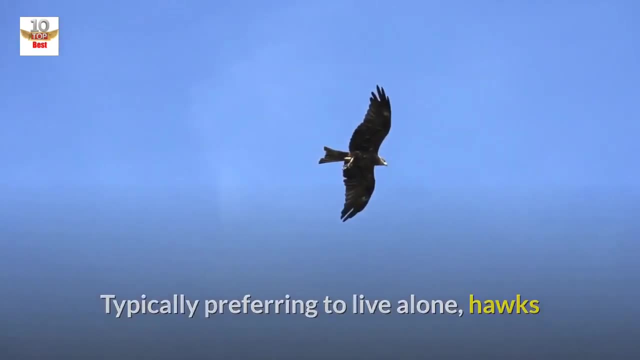 When hawks flock, it's called a kettle of hawks. A kettle might contain thousands of birds, depending on the type of hawk and the time of year. Typically preferring to live alone, hawks that migrate take advantage of large groups to help find warm wind currents, known as thermals. 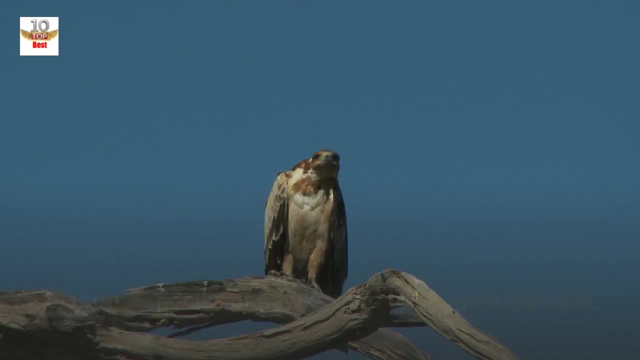 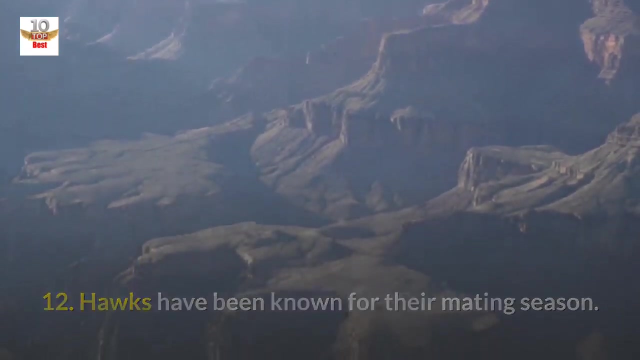 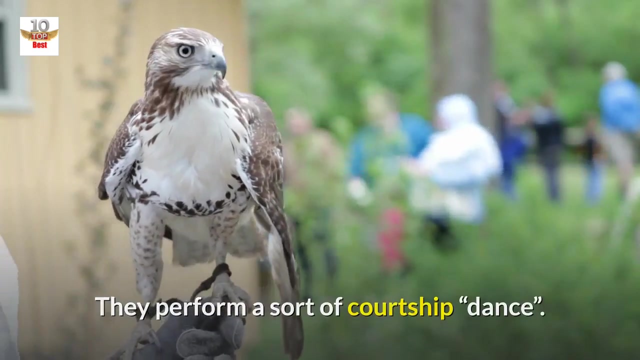 11. Some species of hawks tend to be monogamous, staying with the same mating partner their whole lives. 12. Hawks have been known for their mating season. The method this animal uses to reproduce is different from most. They perform a sort of courtship dance. 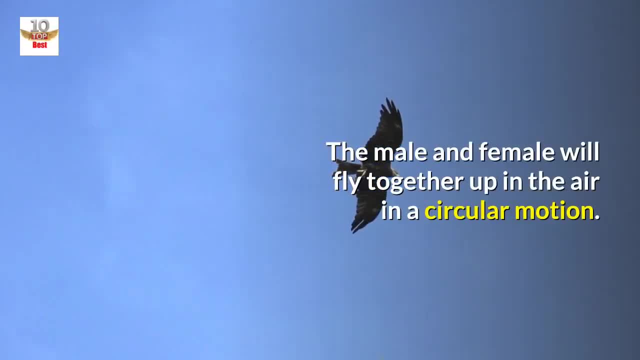 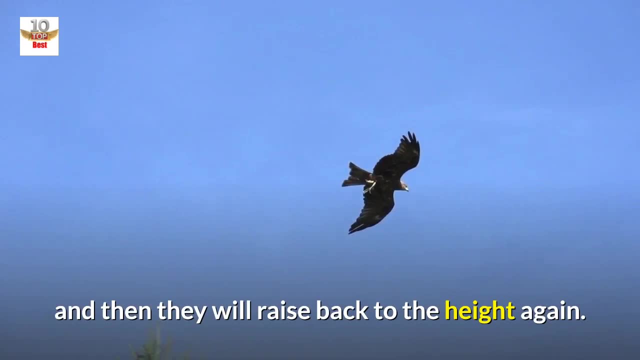 The male and female will fly together up in the air in a circular motion. Once the two get to a certain height, the male will dive toward the female and then they will raise back to the height again. The two birds will repeat this until finally the male latches onto the female and they 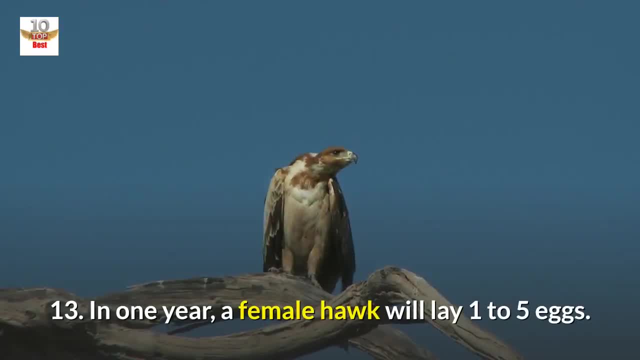 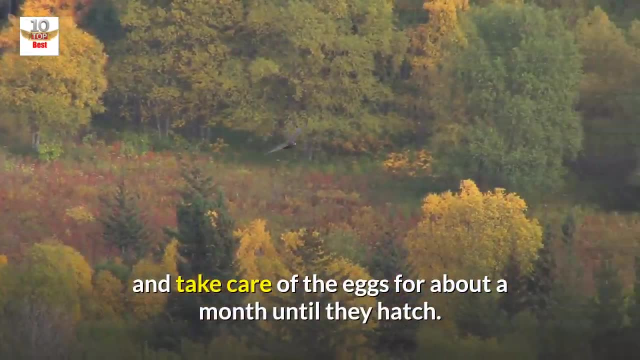 begin to free fall down to earth. 13. In one year, a female hawk will lay one to five eggs. 12. Both the male and the female will cater and take care of the eggs for about a month until they hatch. The male and the female will also create their nest before the mating season and will improve. 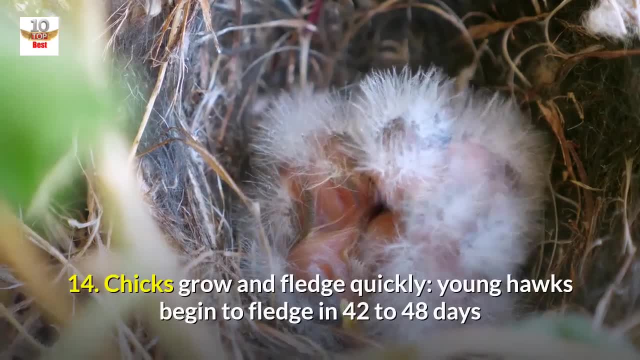 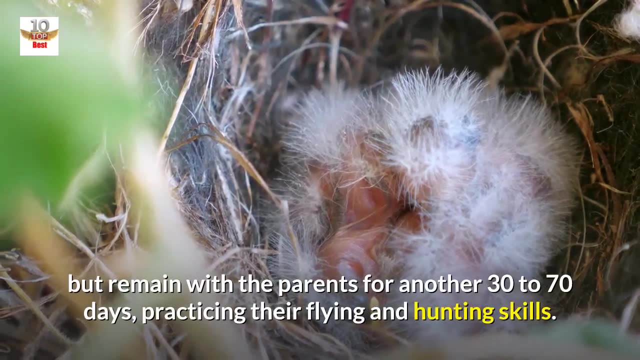 it together during the nesting season 14.. Chicks grow and fledge quickly. Young hawks begin to fledge in 42-48 days, but remain with the parents for another 30-70 days practicing their flying and hunting skills. 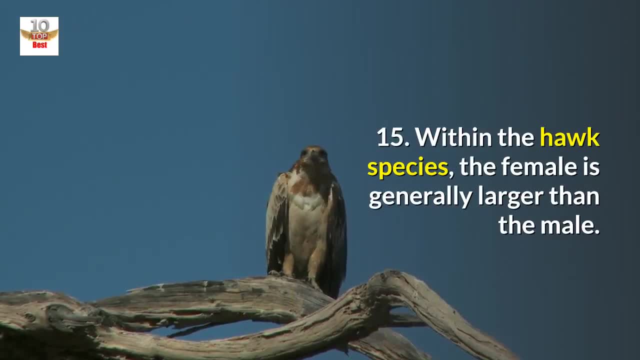 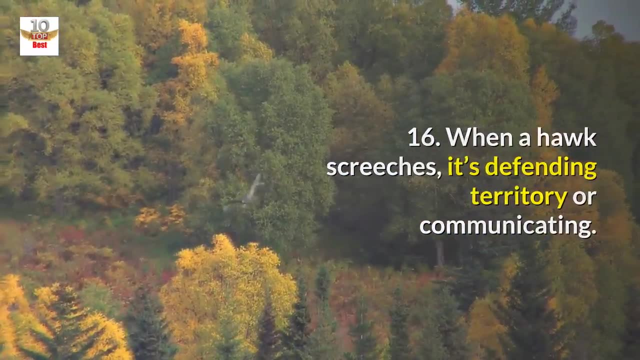 15. Within the hawk species, The female is generally the most active and most active. 14. larger than the male. 16. when a hawk screeches, it's defending territory or communicating. they most often screech in flight. 17 Hawks can see colors like most. 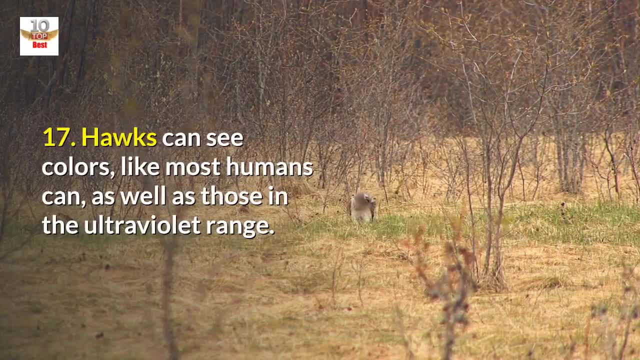 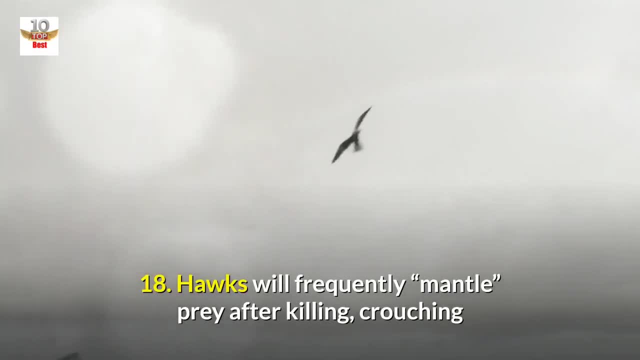 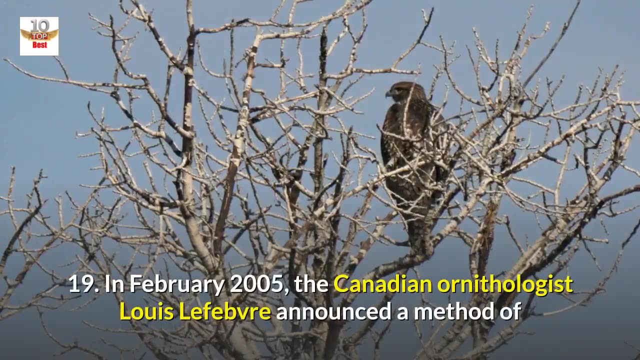 humans can, as well as those in the ultraviolet range. this means that the Hawks can perceive colors that humans cannot see. 18 Hawks will frequently mantle prey after killing, crouching and spreading their wings to form a shield that hides it from other predators. 19 in February 2005, the Canadian 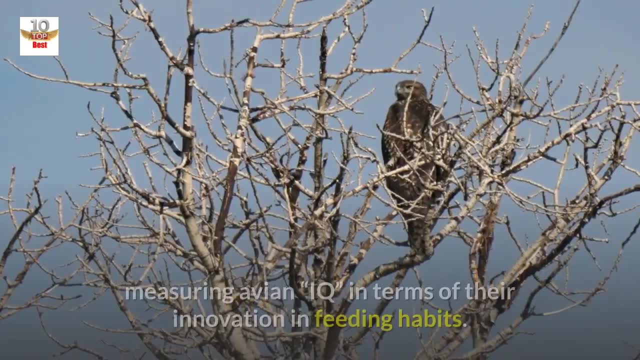 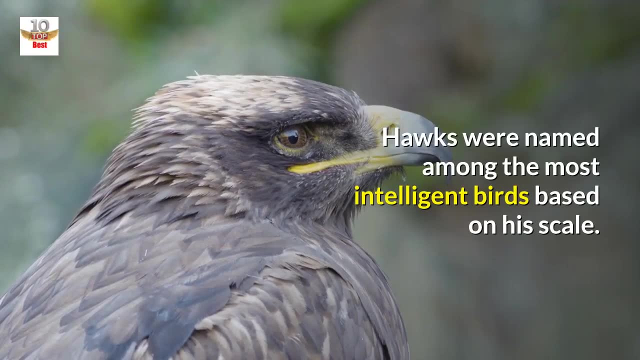 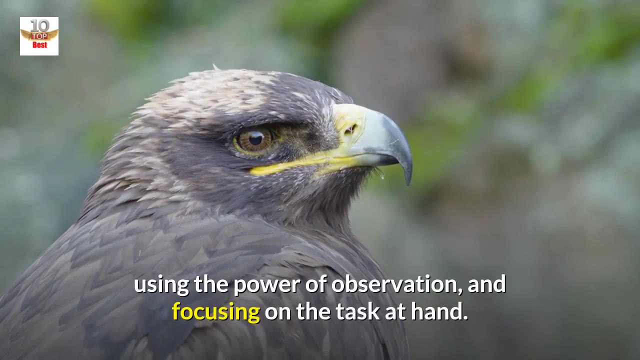 ornithologist Louis Lefebvre announced a method of measuring avian IQ in terms of their innovation in feeding habits. Hawks were named among the most intelligent birds based on his scale 20. the hawk totem provides wisdom about seeing situations from a higher perspective, using the power of observation and